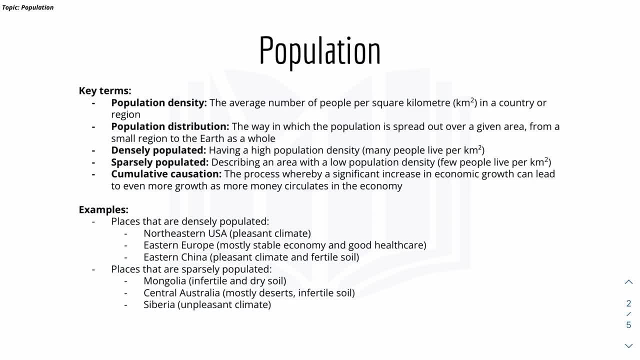 So, starting with population, here are quite a lot of key terms for you to know. So the population density is quite simple or quite straightforward: it's the average number of people per km2, or km2,, and distribution just means how the people or how the population spreads around in a country or an area. 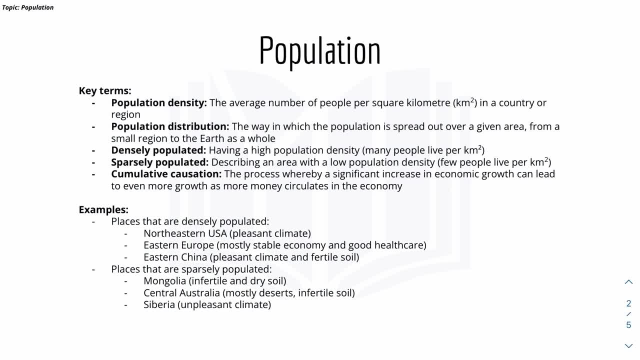 So densely populated and sparsely populated are the opposite. and densely populated is having a high population density- This means that many people live per km2, and sparsely populated just means there's a lower population density. And densely populated and sparsely populated are not to be confused with overpopulation or underpopulation, because overpopulation has to do with the resources in the country, as well as underpopulation. 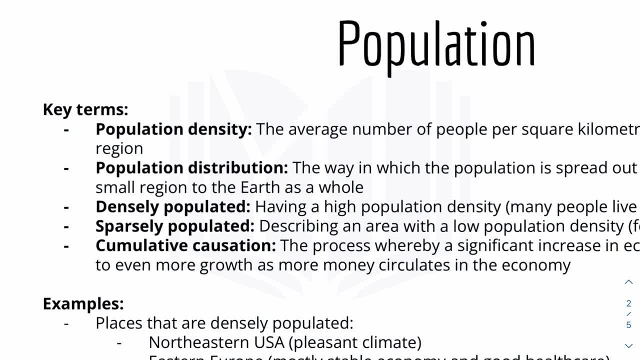 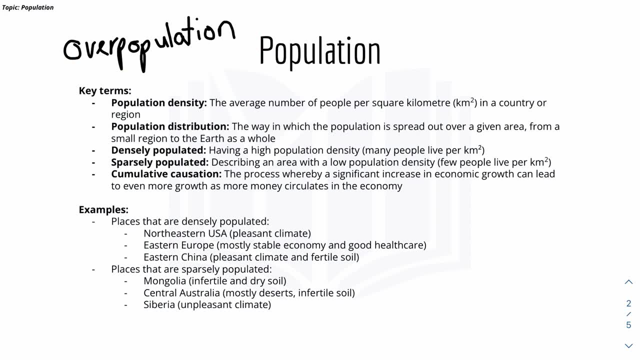 So just to recap, overpopulation. let me just write it down: overpopulation or underpopulation is not the same, because overpopulation means that there's too many people in the country to utilize the resources in the country, so it just means that there's more population, or like more people, than the resources in the country. 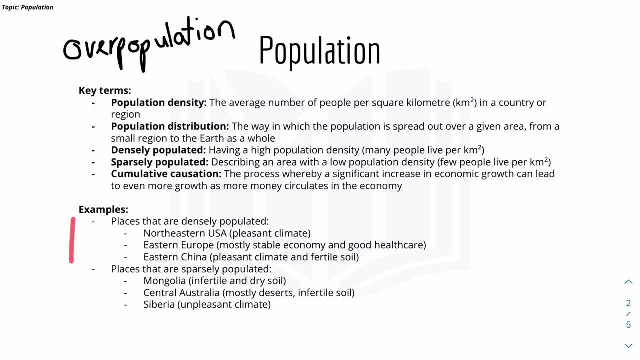 And here are some examples of places that are densely populated and sparsely populated- And densely populated include the Northeastern USA, because there's a pleasant climate, Eastern Europe and Eastern China, And the opposite of that would be sparsely populated. 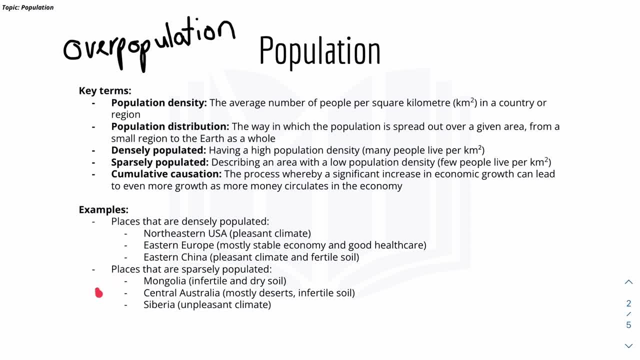 Which, for example, is like Mongolia, Central Australia or Siberia, And there's a pattern that you can see whether a country or an area has a densely or a sparsely population or like populated, And you can look at whether they have a good climate, good healthcare, good economy or like, let's say, infertile soil or unpleasant climate. 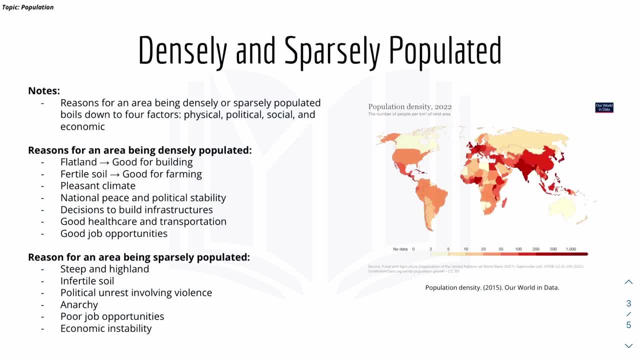 And here we have more notes on densely and sparsely populated. So here's a note: The reasons for an area being densely or sparsely populated. It boils down to four factors, as I mentioned. There's the physical side, the physical factors, political, social and economic. 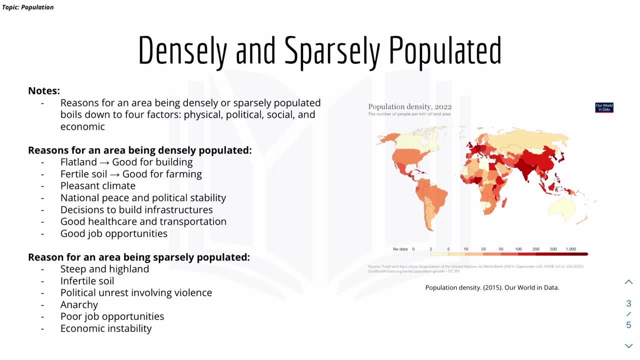 So here are some reasons for why an area is densely populated and sparsely populated. So we have some physical factors, for example, flat land in a densely populated area and fertile soil, as well as pleasant climate, Which means that it's quite nice to live there and you can build a farm in that area, which promotes population growth. 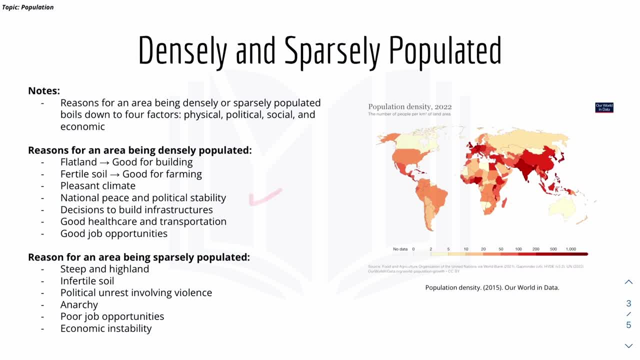 As well as there's a national peace and political stability And there's a good infrastructure, which means that the country is quite stable and people would move into those countries, because those countries have a lot of poor factors. And, moving on to the social and economic, there's also, of course, good healthcare and good job opportunities, which means people would move to those countries or those areas. 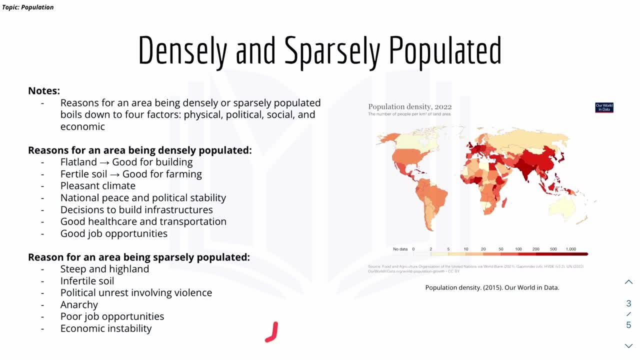 And the opposite of that: sparsely populated. there's some physical factors which is quite important, basically the opposite of these factors. so, like this has flat land and the opposite of that would be steep and infertile soil. there's political unrest. 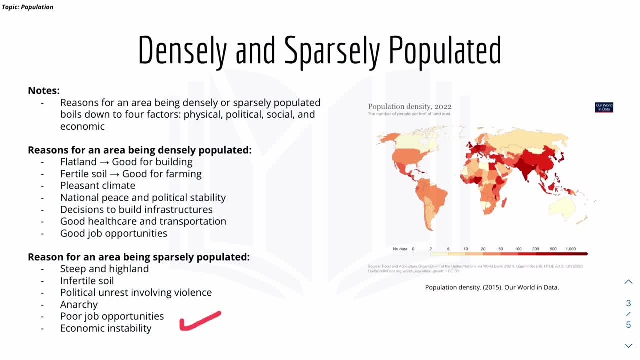 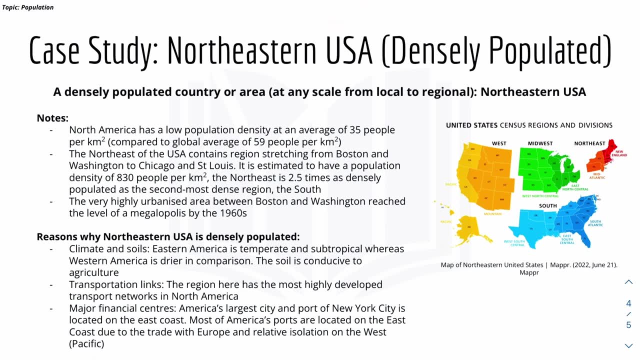 involving violence and there's poor job opportunities and economic instability. so here's the first case study, which is a densely populated country or area at any scale, from local to regional, and we'll look at the northeastern United States of America. so here are some notes. so the area, like the North America, has a 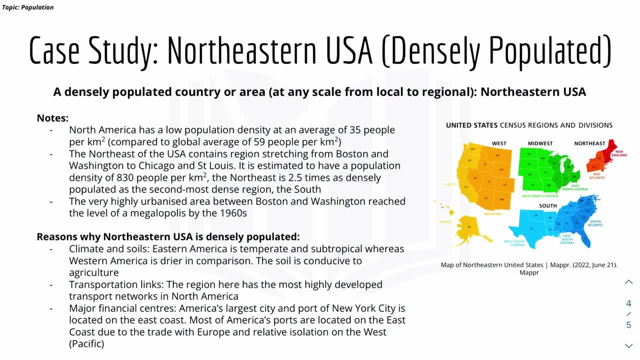 low population density at around 35 people per kilometer squared, compared to the global average of 59. but the northeastern USA, which we'll look into right now, has a density of 830 people per kilometer squared, and the north east of the USA contains regions stretching from Boston in Washington to 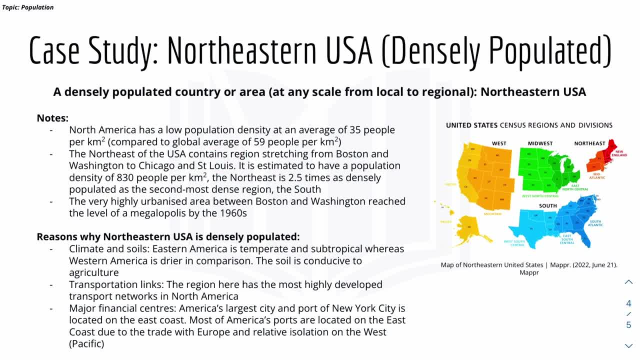 Chicago and st Louis right here. so, as you can see here, this map right here of the United States, that's the West USA, Midwest, South and the North East, is right here and here are some reasons why the northeastern USA is densely populated. so, number one, they: 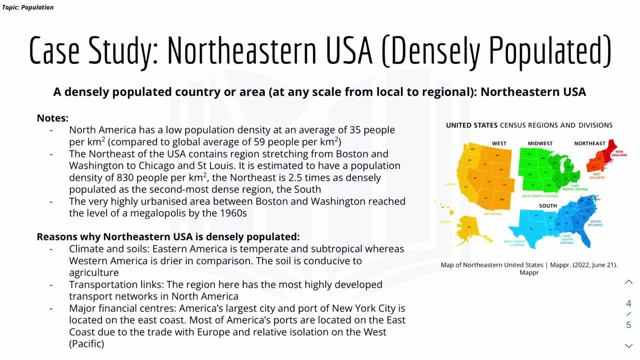 have good climate and soils and the temperature is quite nice compared to Western America, which is drier in comparison, and the soil is fertile for agriculture. so people move to those areas to, let's say, farm or to, like a, promote growth, and here's transportation links. the region here has the most. 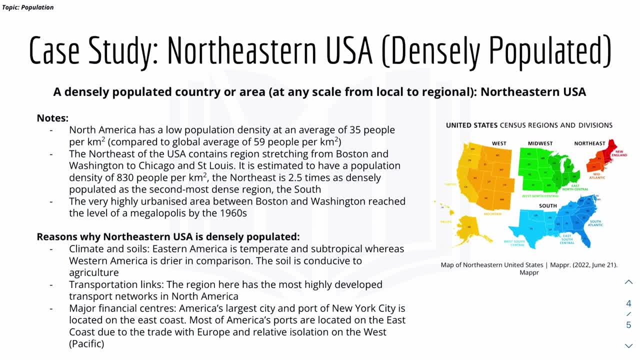 highly developed transport networks in North America because there are quite some important cities in the North East America, so that's why the authorities decide to build good transportation links. and the third point: it's a major financial center in the North East America and America's largest city, and. 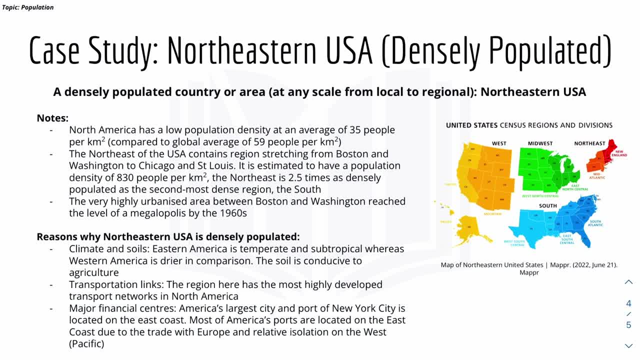 port of New York City is located on the East Coast and most of America's ports are located on the East Coast due to the trade with Europe and relative isolation in the West, because the West right here, because these parts are like this region- right here is the Pacific Ocean, whereas this right here, you can't. 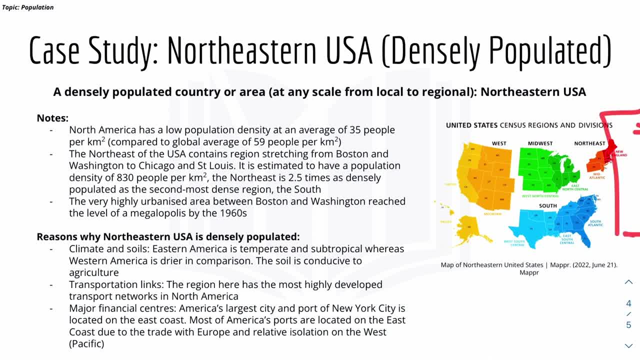 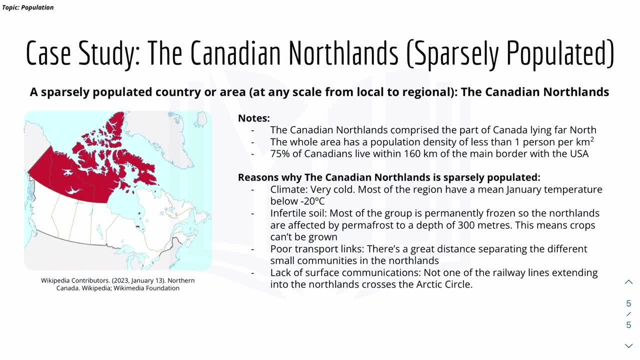 see on the map, on the screen, but it's Europe right here, if you know your geography quite well. and lastly, we have a sparsely populated country or area at any sphere, from local to regional, and we'll look at sparsely, which is the 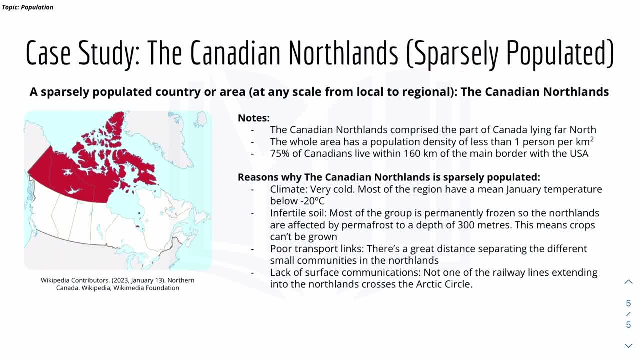 Canadian Northlands. so we mentioned about the USA just now, which is down here, and the Canadian Northlands is basically the Canada right here and above right here. so the Canadian Northlands comprise the part of Canada lying far north and the whole population density in the whole area has 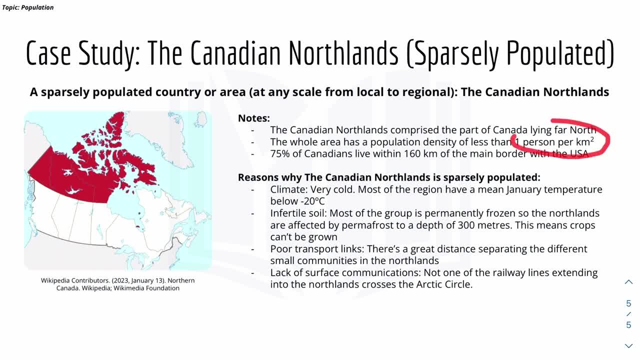 a population density of less than one person per kilometer squared and, if you remember from the previous slide, the global average is 59 people per kilometer squared. so 75% of the Canadians live within 160 kilometer from the main border with the USA, so there's quite a lot of people living. 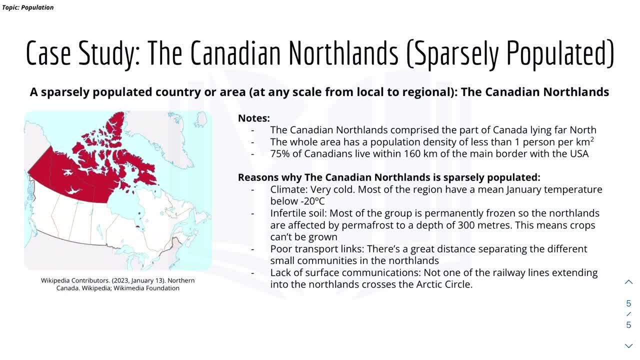 like here, because these are the main cities and here are some reasons why the Canadian Northlands is very sparsely populated. so here we have some physical factors, which is, for example, climate. it's a very cold in the Canadian Northlands because it's so far up north and most regions have a mean January. 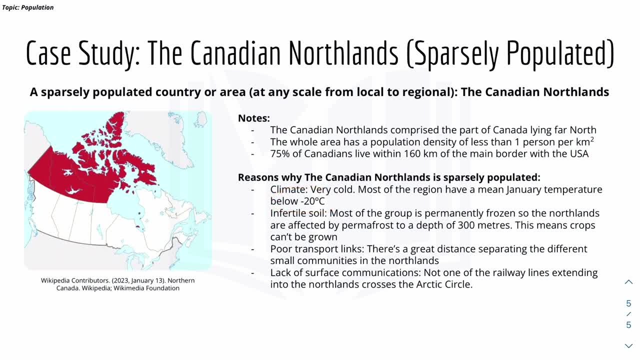 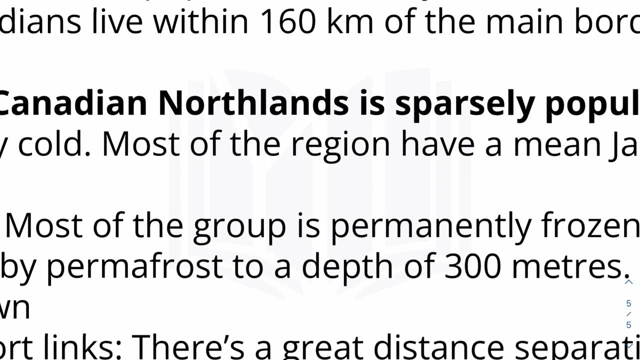 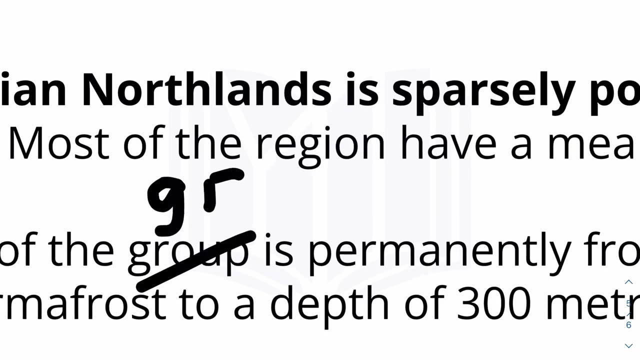 temperature of below minus 20 degrees Celsius. and because it's so, it's so cold and it's like minus minus 20 degrees Celsius, the soul is a very infertile, which means that most of the ground- sorry, this is meant to be the ground, not the group- most of the ground is permanently frozen. so, sorry, yep, so. 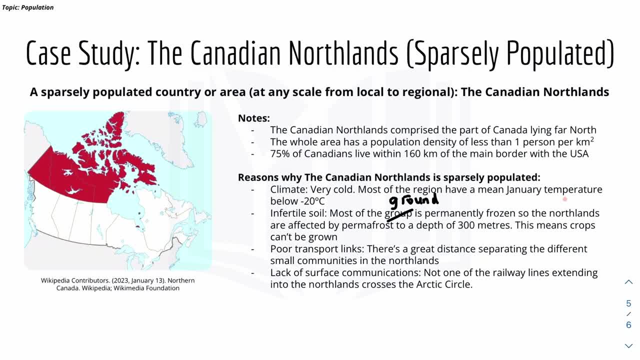 because it's so cold, most of the ground is permanently frozen, so the Northlands are affected by permafrost to a depth of 300 meters, and it's quite deep. so it's that's why that the crops can't be grown and that's also per transport links in the Canadian Gotham as a great decent separating the